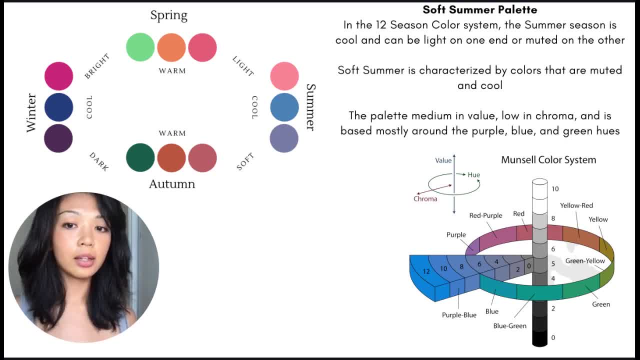 So you might hear this season referred to as summer autumn, in between summer and autumn, because both soft summer and soft autumn share the dominant trait of softness, except summer is cool and soft autumn is warm. So here's a little diagram showing you the different traits and different cooler, warm temperatures that drive the 12 season. 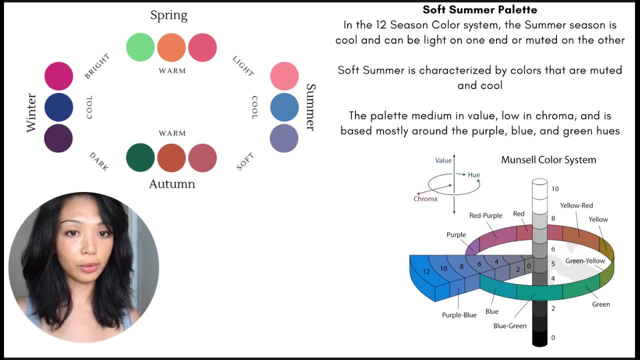 color palette, and I can get into that more in a separate video. Another thing to note or to be aware of is the Munsell color system, which basically identifies colors or breaks colors down into three traits, The first one being value. So if you look at this little pole in the middle, 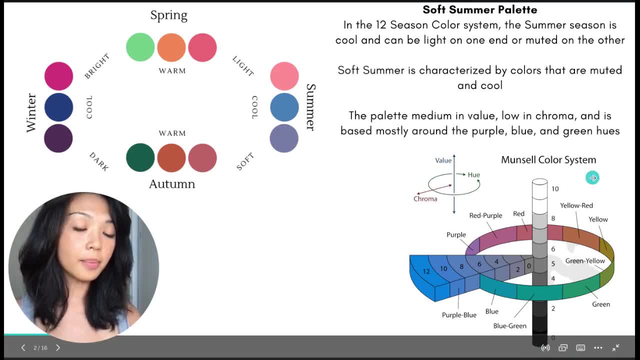 with the numbers 0 on the bottom and 10 on top. these are values, grades of black to white. So if you have high value, you can see a color that has a lot of white to it. Lower value has a lot of. 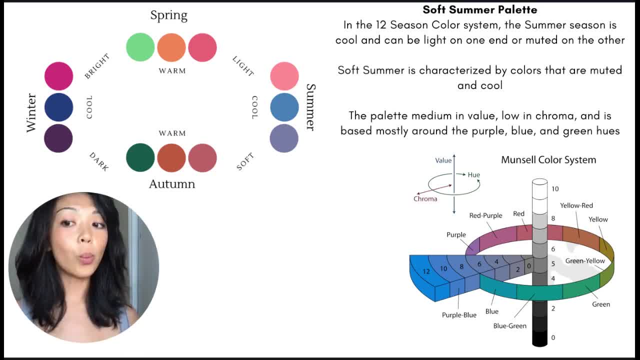 black to it And medium value has a lot of white to it. So if you have a color that has a lot of white to it, medium value tends to have more of a gray tone to it. These colors in the middle are medium value, So they're not at the extremes. Another way to classify color is chroma, So you 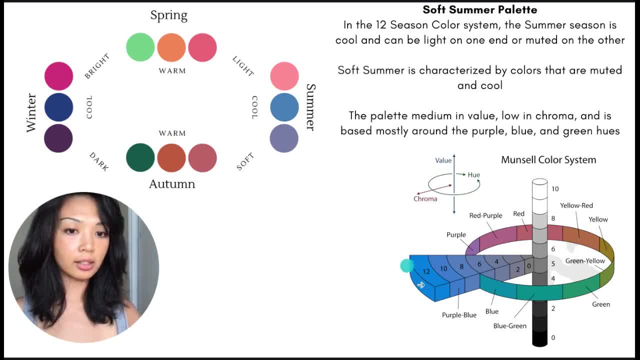 can see all of that here in this little kind of pizza slice. So chroma can be high or low, just like value. Low chroma is less saturated, It has less intensity and pigment to it. And high chroma color has that saturated, almost pure tone. 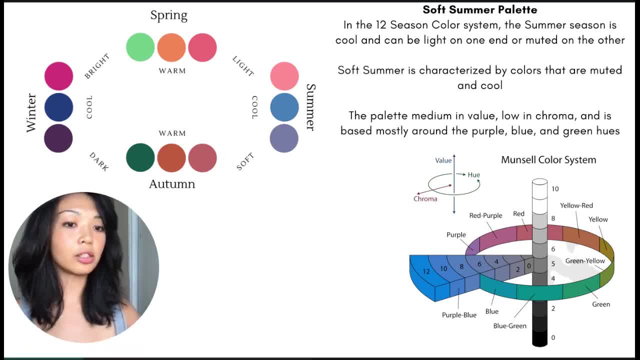 to it. So you're not getting a lot of gray mixed into it. You're not getting a lot of the values mixed into it, It's more of a pure saturated color. And then you have hue, which is another term for actual color, So the colors of the color. So if you have a color that has a lot of white to it, you can. 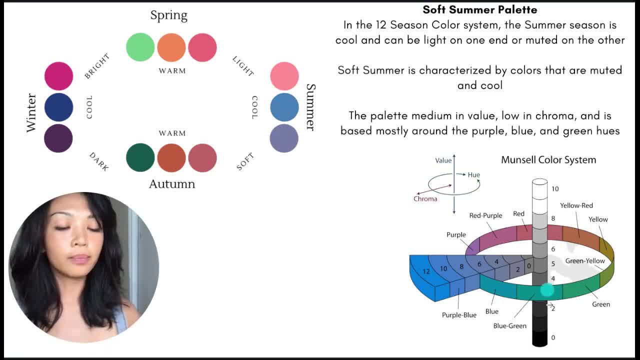 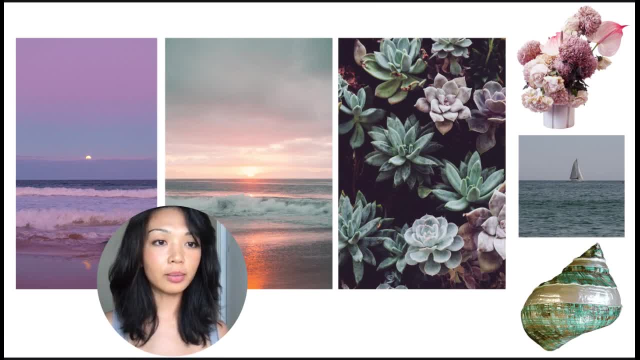 see that that's going to be a lot of pink, which is the color of the rainbow, And the cooler colors tend to be blue, green and a little bit of purple. So just to make things a little bit more fun- because there's so many different soft summer palettes that you can look up online- And just a reminder: 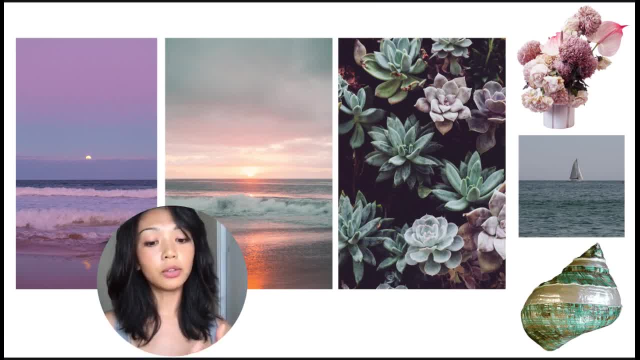 these palettes are based on probability. If you are a soft summer, the colors of a palette will most likely look good on you. maybe not in equal degrees, But the probability that the colors of your color will look good on you is a lot more than just the color. So if you have a color that has a lot of pink, 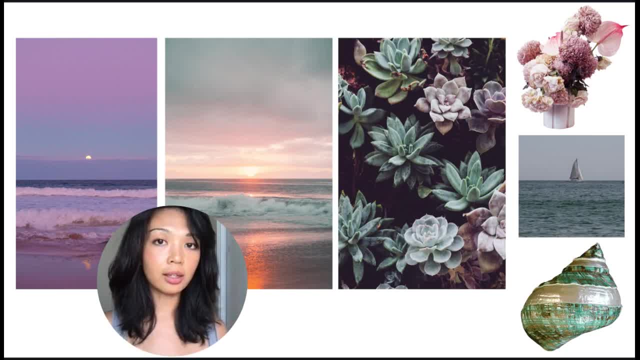 they will really harmonize with your own shading is high. that being said, the color palette is not an individualized, customized fit, so you have to take that into consideration. there are some colors that won't look good on you, and there's some colors from other palette seasons made by other 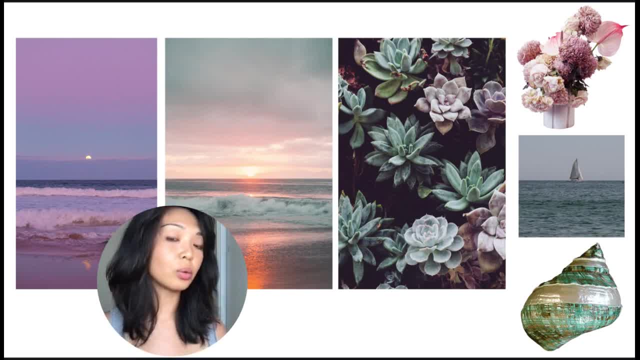 individuals that might work. so stay open and don't look at the system too rigidly now that that is out of the way. here just some example images that i think really represent the the feeling and the color of the soft summer season. soft summer is muted. there's this hazy, diffuse quality to it. 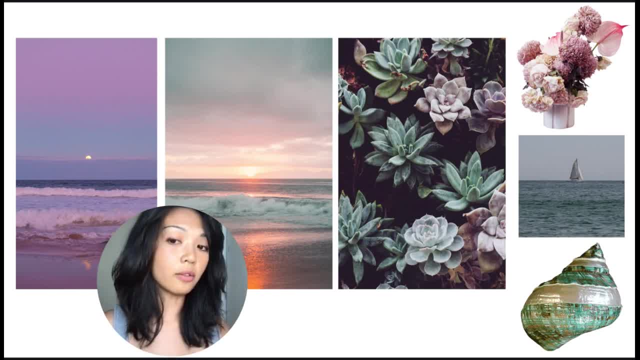 and there's this coolness to it- all of the colors as well. it's not super cold, it's kind of in the middle. there's some colors in the palette that can lean slightly warm, but usually quite cool. a good way to remember the soft summer palette is to think of succulents that can withstand the summer heat but retain. 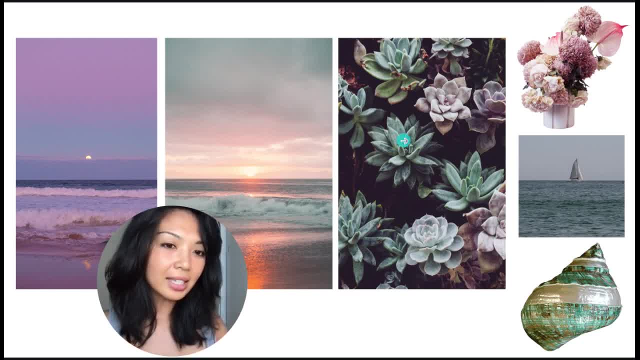 their coolness and they have this kind of slightly misty, frosty white covering on the leaves. that should give you a good way to characterize this season. so look at misty, hazy sunsets and sunrises, succulents, seashells, sea glass, soft silvery ocean waves. 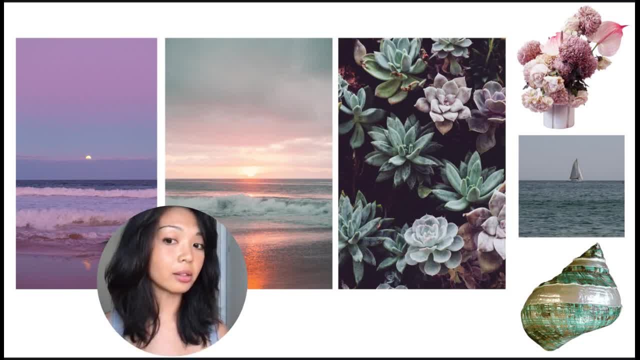 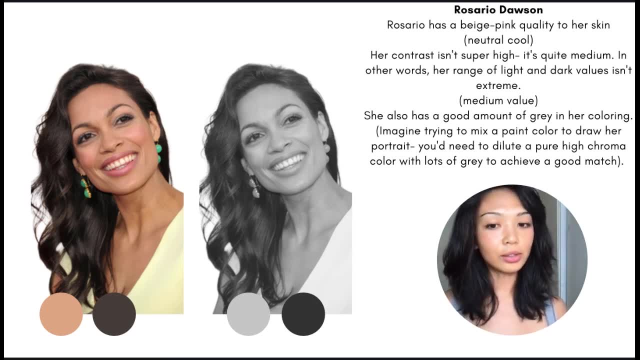 muted flowers, dried flower petals, nothing bright, nothing too saturated. it's a very gentle, hazy season, all right. so now that we've gone over a little bit of the background on the palette, let's look at some lovely examples. the first example is rosario dawson. 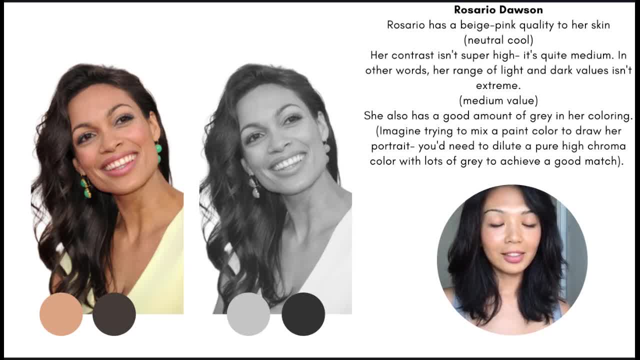 beautiful rosario dawson. um, i haven't seen her in a while, except for in the mandalorian, but she is absolutely beautiful and i think she's going to be one of my favorites for this season. so i'm going to go ahead and show you a little bit of a look at her. 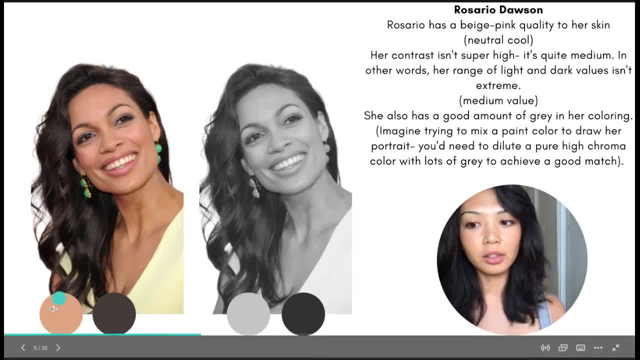 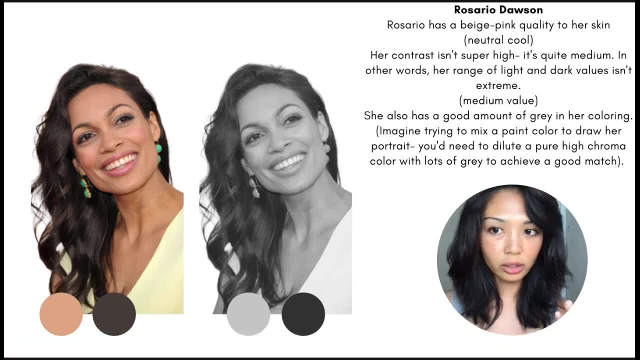 so let's look at her skin tone. so i've pulled these two little color swatches of her skin tone and of her hair just to give you um kind of a closer look at what i'm referring to. so if you look at her skin tone, she has like a sort of beige, pink tone to it. there's nothing. 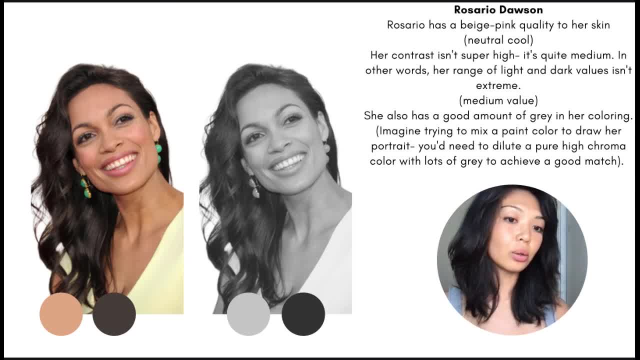 super warm about her skin tone, so she doesn't have undertones. it's like walnuts or honey, um, or like an orangey hue to her skin. she has a kind of cooler, slightly neutral toned skin, um, and her hair is dark, yes, but there is a coolness to it. it's like 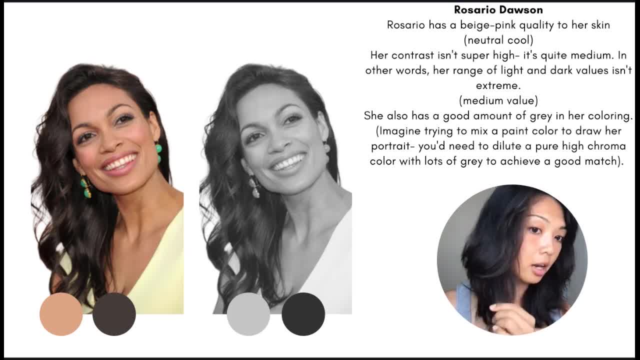 slightly charcoal-y, ashy kind of like my hair. my hair is not jet black, it's not blue black. there is a soft gray tone to my hair. i see that in rosario as well, so she's definitely cool toned and she's very soft and muted in her coloring, so there's not too much. 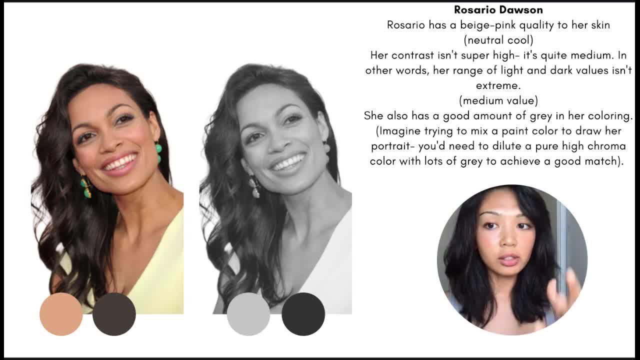 brightness to her skin tone. there's not too much depth. she has this very soft diffuse quality to her skin and her hair. there's something like sharp about her shading and, um, if we look at her in gray scale, her colors range from the i would say three to seven range on the, the value system, so gray. 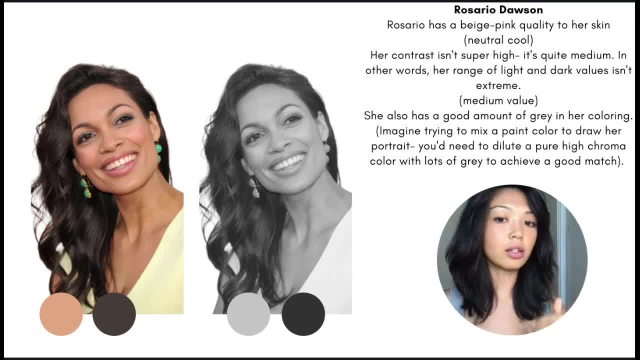 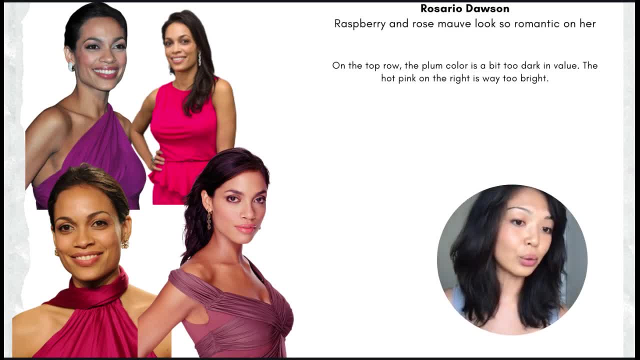 to charcoal, but not white and not black. all right, so let's look at some color comparisons and tie that into her color characteristic. so on the bottom, we have, in my opinion, two colors that look absolutely stunning on her. a color will look stunning on you if it makes your skin. 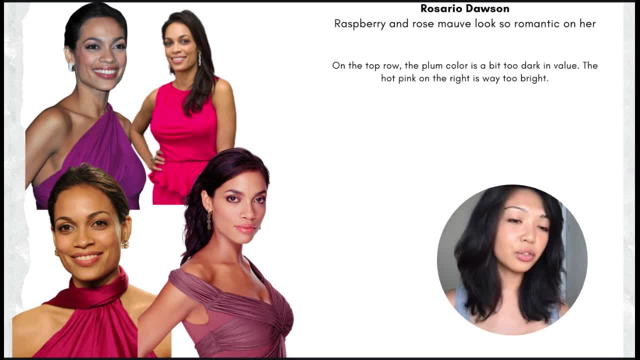 look even more healthy and radiant. and there's different ways for skin to look radiant. it doesn't always have to mean super bright or super sharp. radiant skin can also look creamy, it can look buttery, it can look smooth. there's many dominant characteristics, many different types of glows, so 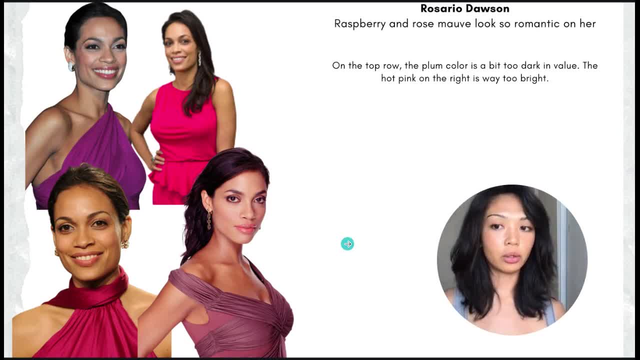 that is a good sign that a color really works for you. and another sign that a color really works for you is that it isn't overpowering you. it's kind of harmonizing with your skin and hair tones so you can appreciate the color but more so you can appreciate its overall kind of. 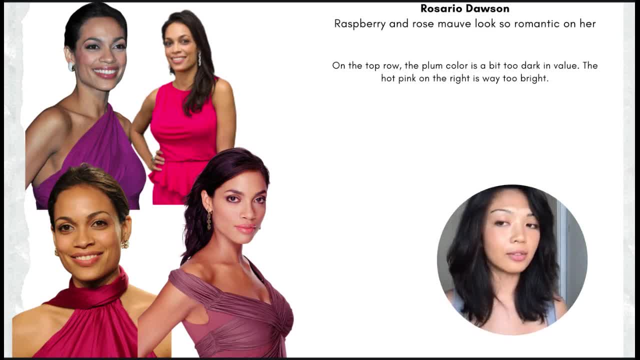 synergy with your hair, your own silhouette and face and hair. so this pretty slightly muted raspberry in a material that's not too shiny makes her skin look phenomenal. and here is this: like dusty, like mauvey pink, and her eye shadow here is also kind of the same color and she just looks so glowing now on. 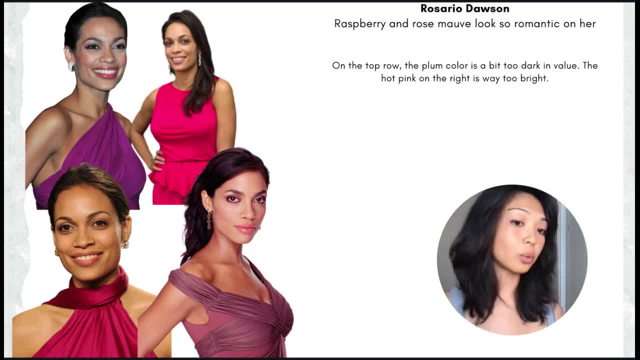 the top. um, i don't think these colors work as well. so here this purple is a little bit more deep, i would say it has more of the black values to it, so you have less gray and more of that darkness, that depth to it, and i think it kind of overpowers her. um, and on the right, this is a very 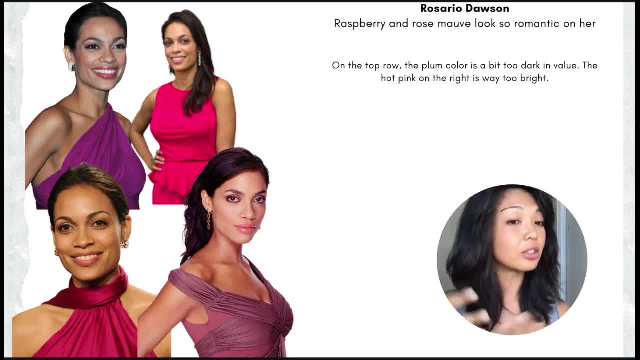 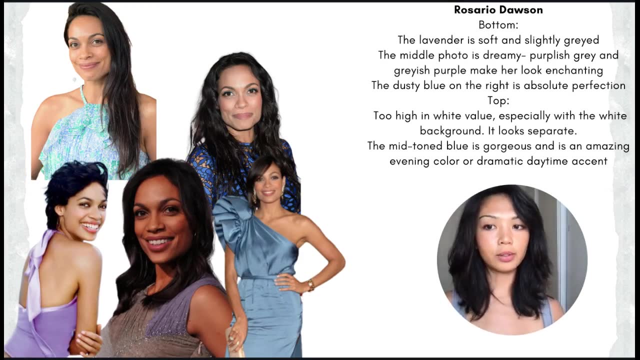 bright color and kind of opposite of softness, brightness, um, and it just really takes over. so i see the color and i don't see rosario. all right, so let's look at some gorgeous blues and purples. so here this lilac color looks very. 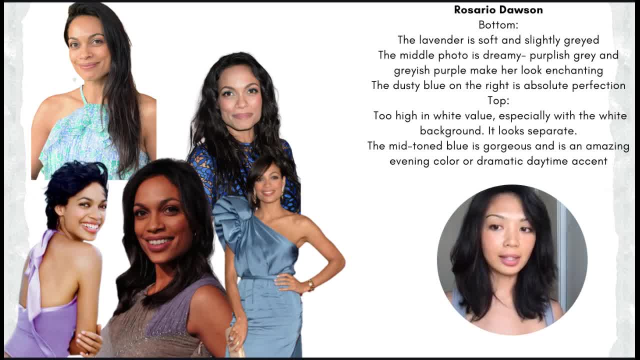 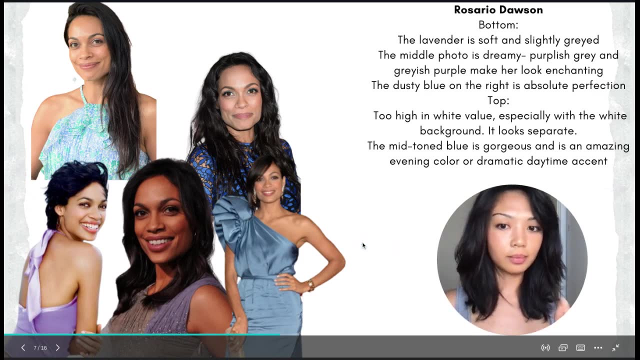 heavenly on her. she looks so whimsical and light and radiant. this gray and lilac, pairing with a slight twinkle of the, the metallics underneath, also gorgeous blue. this like dusty, almost teal blue is, i think, so gorgeous on soft summers. it's the power color. 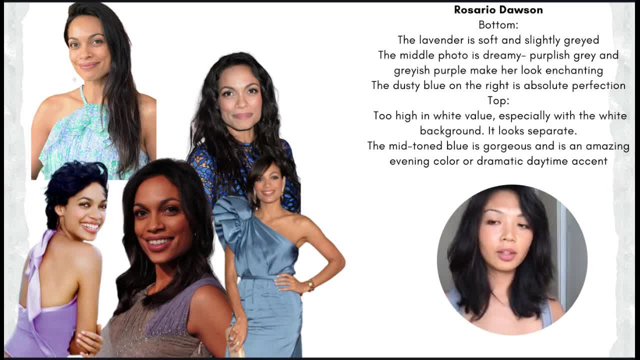 or at least the power of blue for many soft summers, all right. so total opposite of that. this blue and green with a lot of white here is just very bright and it kind of washes her out. so because of color contrast, you're seeing how bright and light these greens and blues are, and then you're seeing 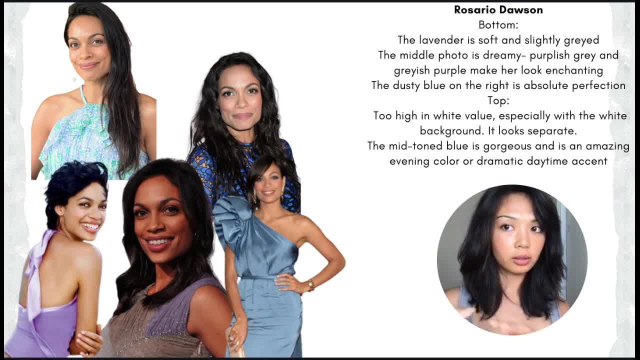 her skin and her hair, which is much more soft and muted, so it does tend to overpower and wash her out. now here on the right, um, there is a black outline across or around all of this gorgeous blue, but you have to remember that during night time you can really play with. 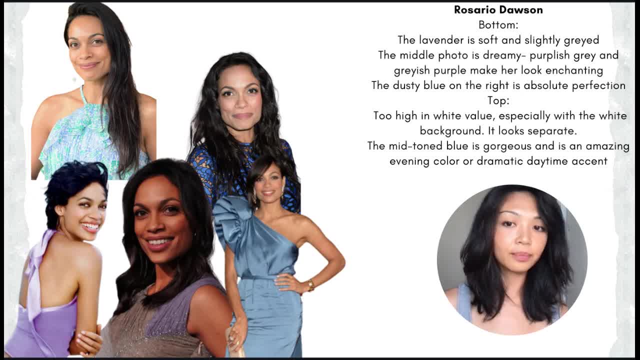 colors that are a little bit more intense than your daytime palette, and because of the blue, because of the light use of the black outline and because, um, the skin tone does pop out from these translucent sections, the black isn't overpowering, so remember that these rules aren't. 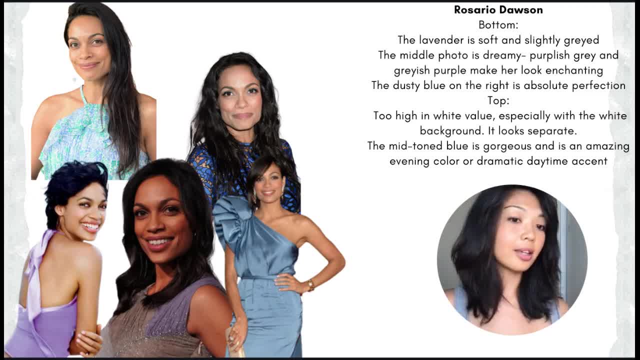 like black and white or rigid. you have to think of these colors and their effects in terms of dominant aspect. what is being exaggerated and is harmony still being upheld? or is it kind of being thrown away? and there's just so much flexibility? all right, so some more beautiful. 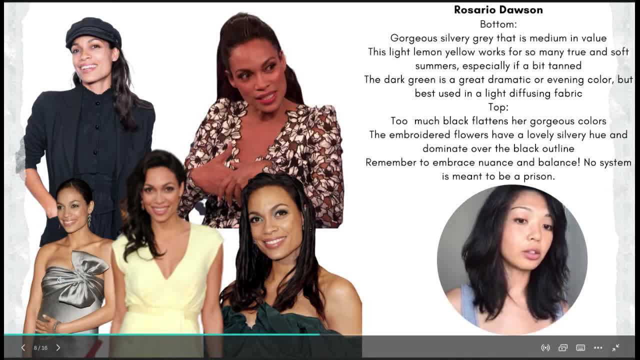 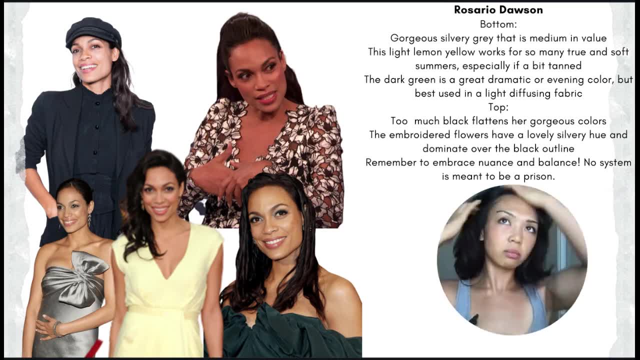 colors: silver, silvery, gray. grays look great on soft summers. i'm wearing a gray dress myself and, um, if gray tends to make you look, i guess, a little bit dead or kind of like a corpse, highly unlikely that you're going to be a soft summer. grays tend to really bring out the 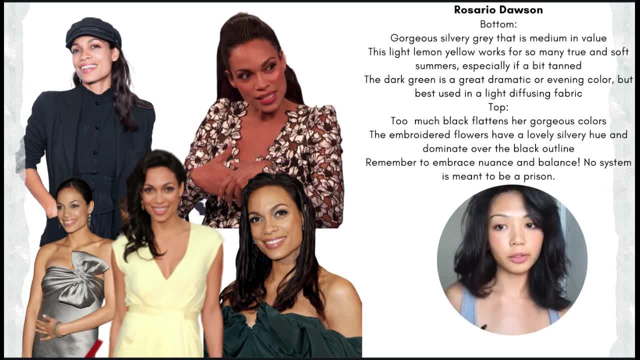 values of the soft summer. so it's not a definite rule but it's probability. here is this gorgeous yellow. it's a cool yellow. so a cool yellow will look less acidic than a warm yellow. so a warm yellow is like like this pen, like sunflower marigolds, um golden yellows. those are going to be warmer. 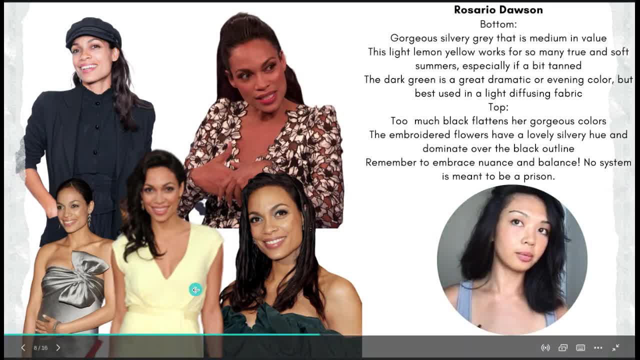 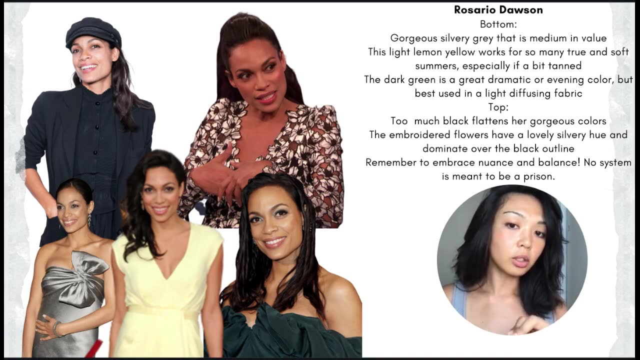 yellows, and these yellows are a little bit more, i would say, subdue. they look like dried flower petals in a way. here on the very right on the bottom, we have this darker green, and this green would look or seem like would be a little bit too deep and dark, but because of the occasion, it's nighttime. 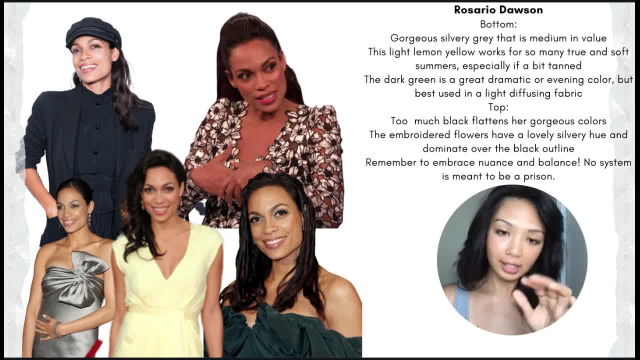 because of the fabric that is just slightly shiny, so this color doesn't look too flat and one-dimensional. and because she has exposed so much of her um decolletage and this deeper color is not like right against her face. it still brings out the beauty of her skin and it's deeper but it. 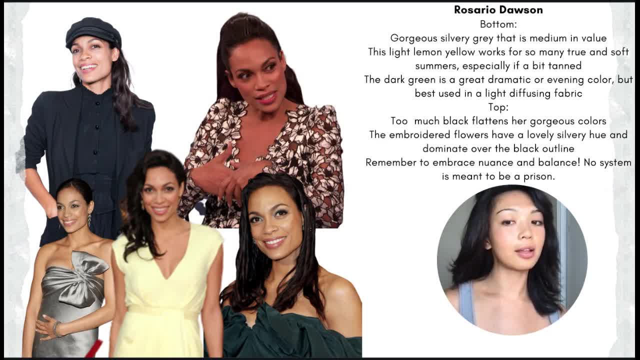 doesn't overwhelm. so again, you can play with many different colors. you just have to know where to place it and at what point. it being so close to your face kind of throws off the harmony. here we have this other very similar kind of dress to the, the blue outline dress from: 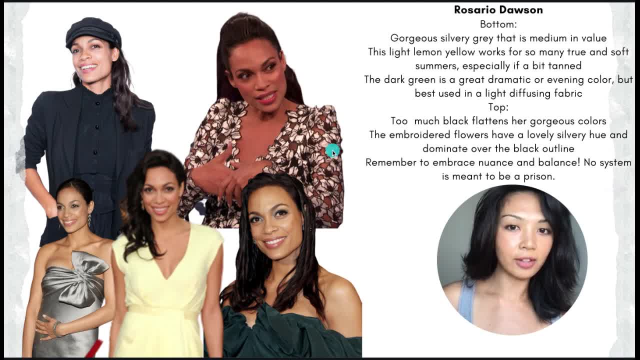 the previous slide, this white, silvery flower with her skin peeking through the transparent regions and thin veins of the black outline. it almost looks like jewelry on her, like she's wearing a beautiful dress of soft pearl or like very soft silver gorgeous. here she's wearing all black. 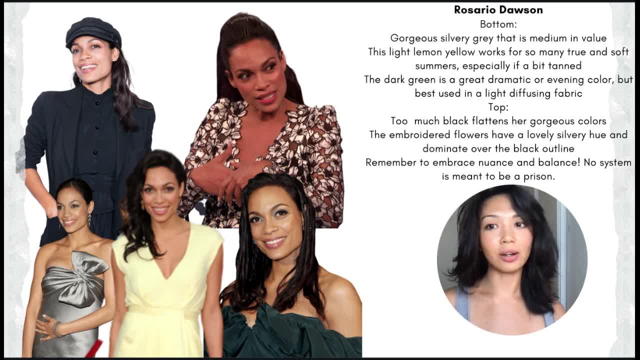 and i just think that it just really flattens and overwhelms her. um, it doesn't really emphasize her natural glow and it's just a little bit provide someKeys that might definitely bring out some of her black wrinkles. or haven't seen a lot of her black wrinkles or jumping into all the black. shapes, but we're just drawing a straight line, you know. but it's going to run me over with the ize way to theipsy for only two seconds. so i did the strive, this one that would probably blow out, because you don't want to mess this one over, so i didn't need to draw it too long. but 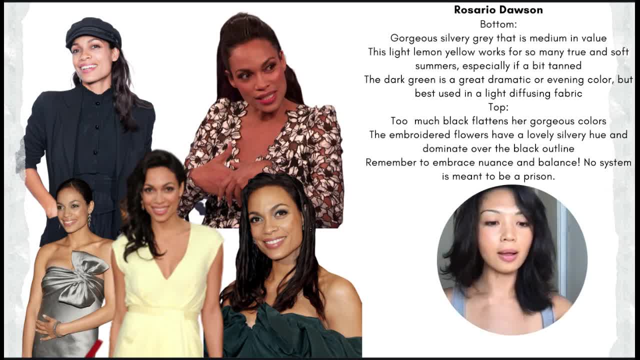 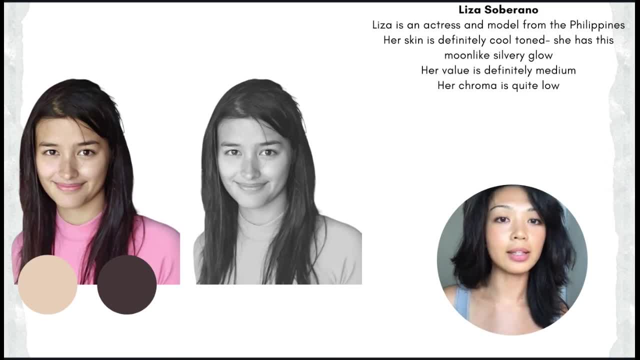 i'll just show you something that i think is very similar, a trick to work this運. a little bit too heavy, all right. so our next example is a Filipino actress. her name is Lisa Soberano and she's really beautiful. she has this very soft kind of. 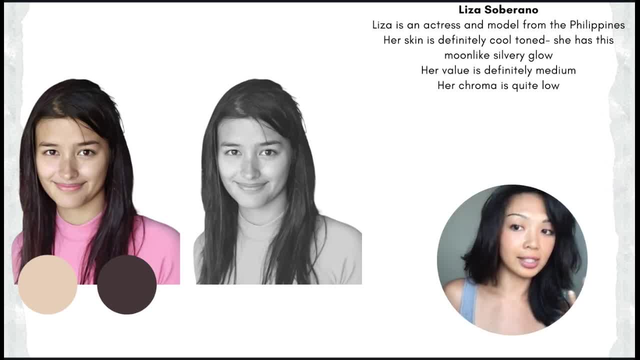 like gray, beige glow to her skin- and I know that sounds really weird to say gray glow, but I swear it's quite accurate for this soft, summer kind of characteristics like a silvery, gray, diffuse glow that's coming from within and she has kind of softly gray undertones to her hair. it depends. 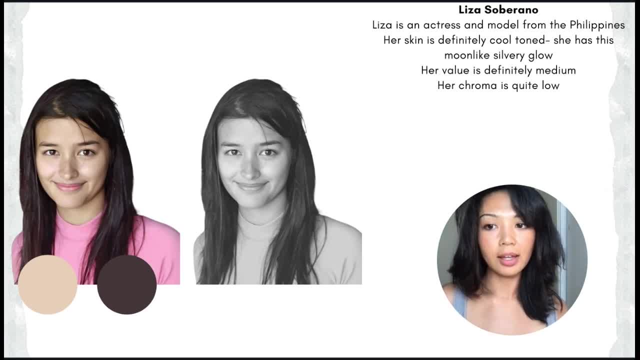 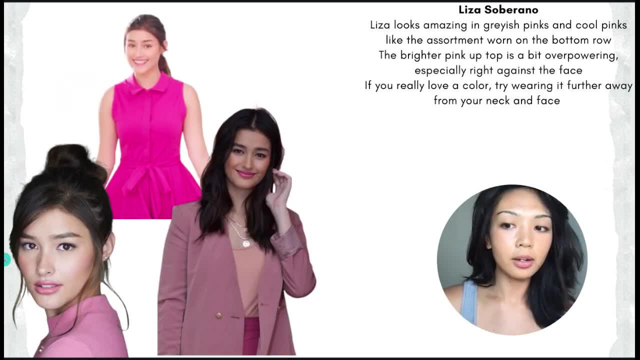 because she kind of switches it up, but she has dark eyes and dark hair, so let's take a look at some of her colors. so on the bottom, here and here, we're seeing so many beautiful pinks that are really grayish pink, or kind of mauve pinks, or muted raspberry pinks, even a little bit of slightly muted rose gold, and 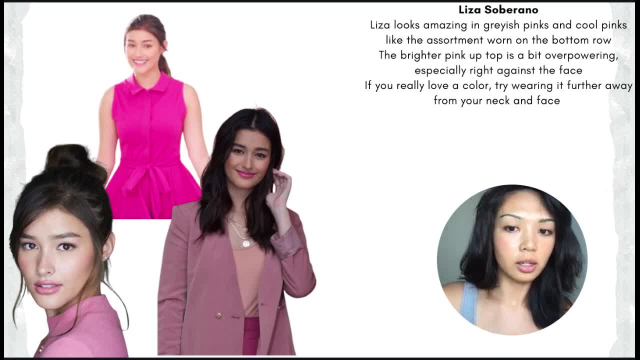 these are all gorgeous colors, especially fun if you pair them with each other, like she's done here. and the finishes of the actual items are also lovely. they're not too shiny but they're not too flat. there's just like that slight pearlescent light diffusion, especially with the cuff here. 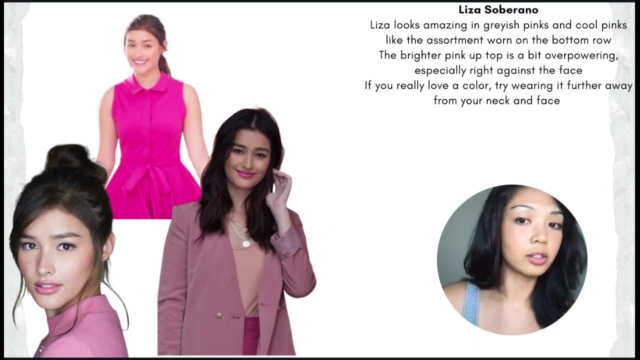 so really lovely colors that bring out her features and they really coordinate with the values or the levels of contrast that she naturally has here on top. just really, really bright. it's just a little bit overwhelming. if you really love a color and it's a little bit overwhelming, try wearing it further away from your face. here are a selection: 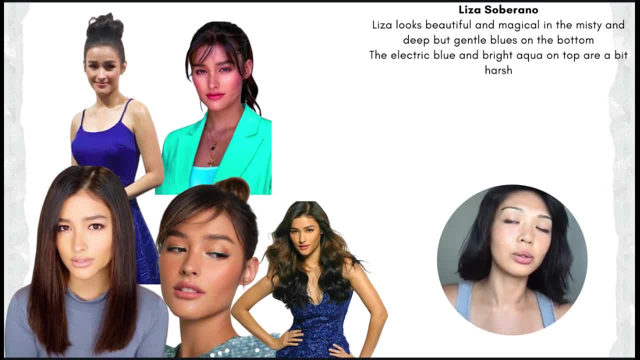 of blues, just like absolutely gorgeous, gorgeous, heavenly blue. so I know I said heavenly a lot, but it's just, I think, a great way to think of this season. it's very ethereal, mysterious, misty, gentle, it's kind of like fairy tale colors. so gorgeous gray blue here. um, here is a deeper blue, but it's. 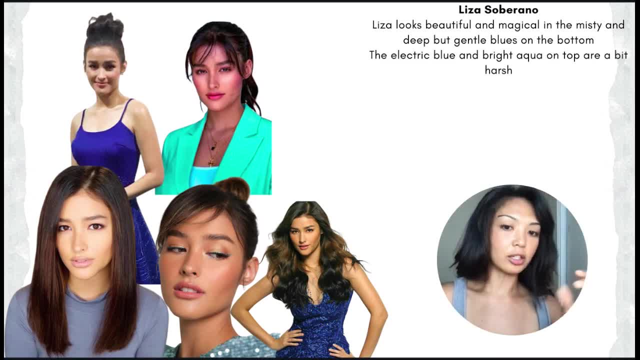 further away from her face and there's this kind of gentle texture to it, so it's not like super in your face. um, she looks kind of like a mermaid in these blues and here on top we have these very sharp electric blues. it's very sharp electric dark blue and this very bright aqua and it just kind of takes over. it doesn't. 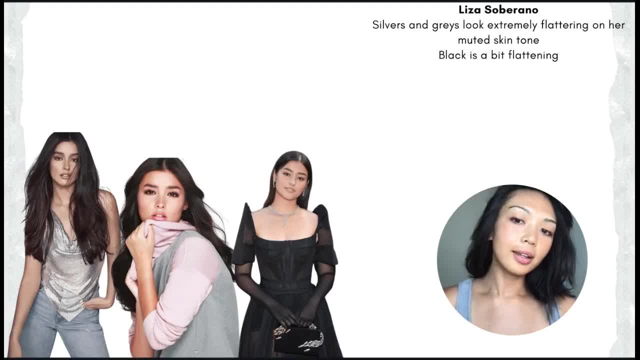 really harmonize with her skin tone. and again, here are some silvers and grays. and just looking at this picture on the left, another good way to tell if you have soft coloring or if you're even a soft summer in some cases. um, it's still like play around with makeup and filters if you look. 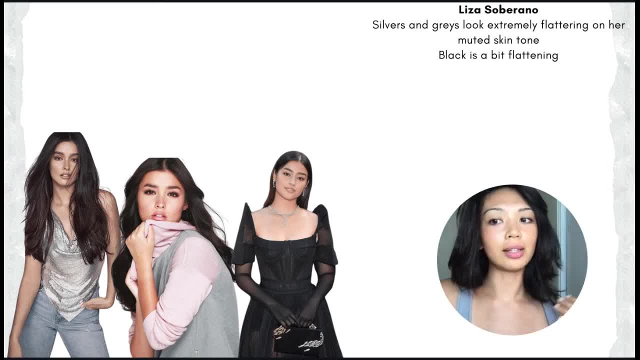 good, even when you lessen the saturation, lessen the contrast and wear makeup that might look a little bit, I guess, like faded on other people. you might be a soft summer like here. her makeup is just very subdued and faded, um, and this kind of makeup might look like kind of like a corpse on. 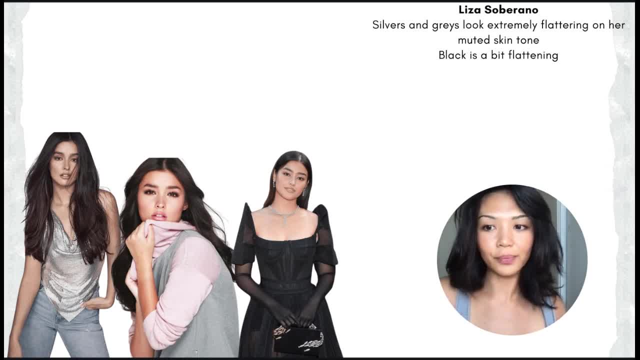 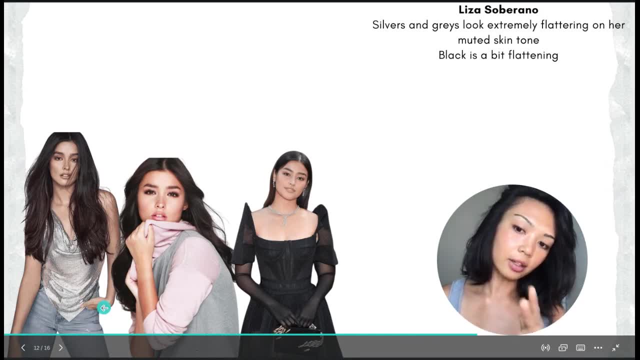 other people, but on her she just looks very sultry. so, um, one kind of strange way to tell. but here gorgeous silvers, nice kind of like silvery blue jeans, pink and gray looks great. and then we have black, and the black just really overwhelms her, even though. 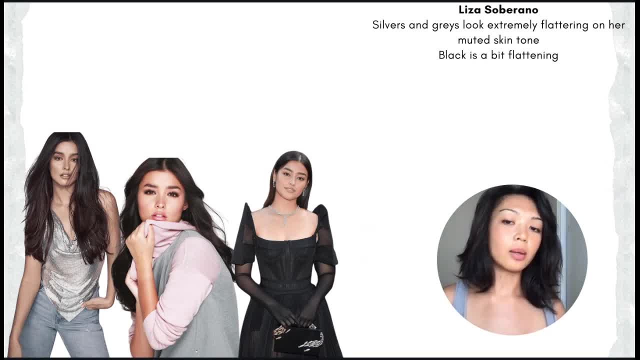 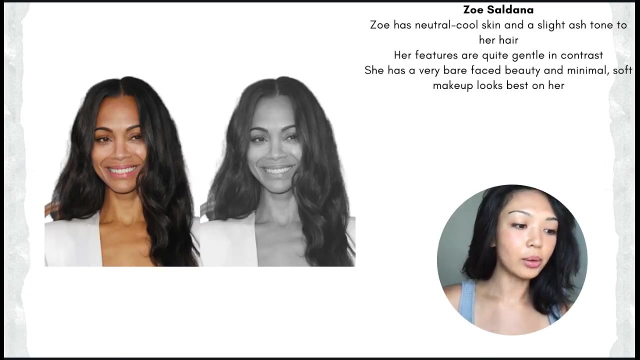 the black is further away from her face, um, it just kind of like steals all the glow from this beautiful woman and it just kind of flattens her. so black tends to overwhelm you, but you're cool toned. look into at least the summer season. and our last example is Zoe Saldana, and I didn't know her name was Zoe Saldana because, um, 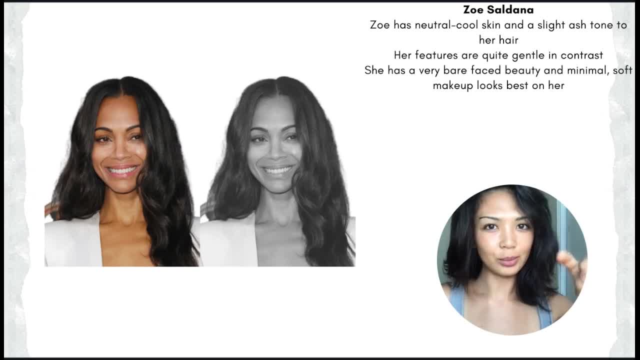 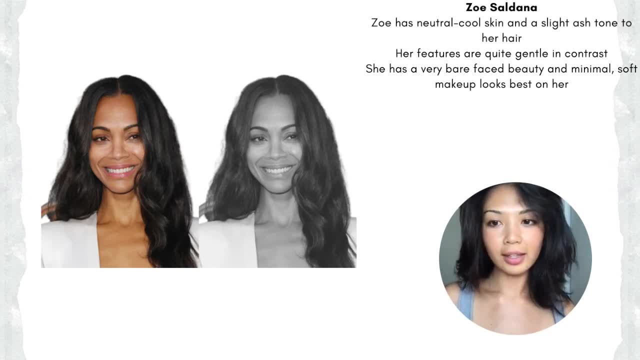 recently on Google search they updated her last name to have the the Enya over her last name. so, um, anyways, Zoe has gorgeous, kind of cool, neutral skin tone, same thing as kind of Rosario Dawson. they have very similar hair and skin tones and very similar contrast in terms of features. they have very gentle, soft features that 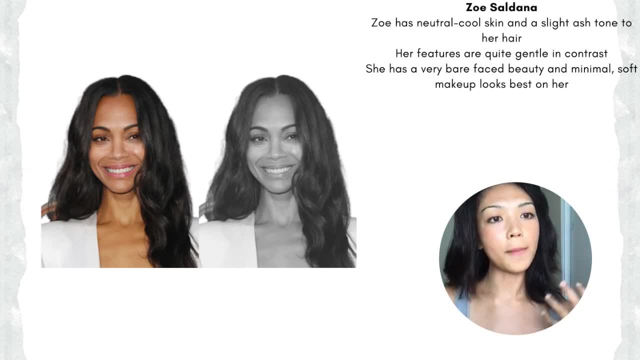 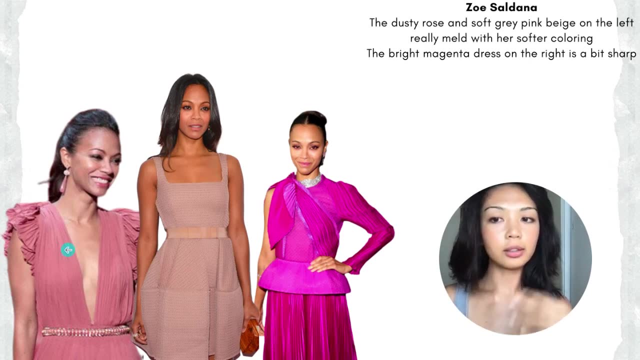 um, kind of blend in their face. they both have that soft, bare face, very fresh beauty. so on the very left here, gorgeous, slightly dusty or powdery pink, here is this lovely gray pink, beige, and those are really great on her and they really work with her softness. but here again this magenta tone which you've seen on the other two examples. it's 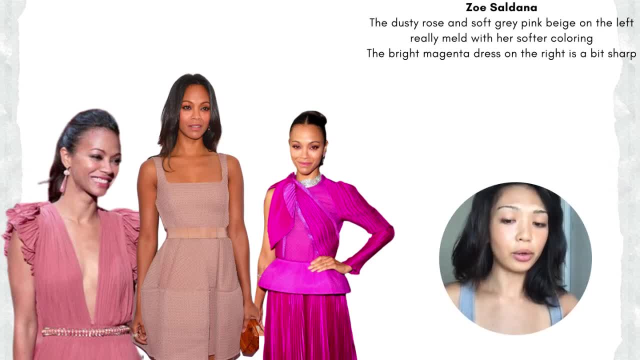 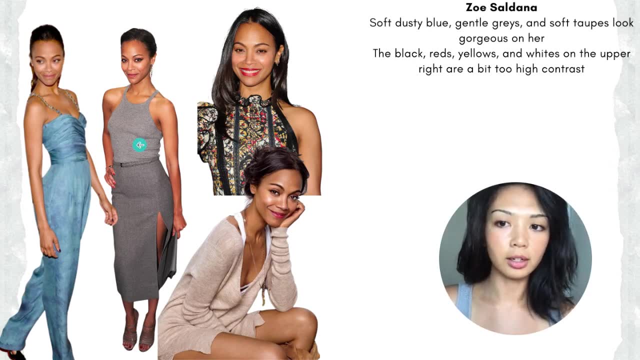 just very bright, very intense, overpowering. here are some more beautiful colors. this just gorgeous, gorgeous dusty blue, here, gray on gray, looks exciting on a soft summer. here is just this lovely understated beige tan, just beautiful. and then here very high contrast: black, the white, the red, the golds, um, that's. and 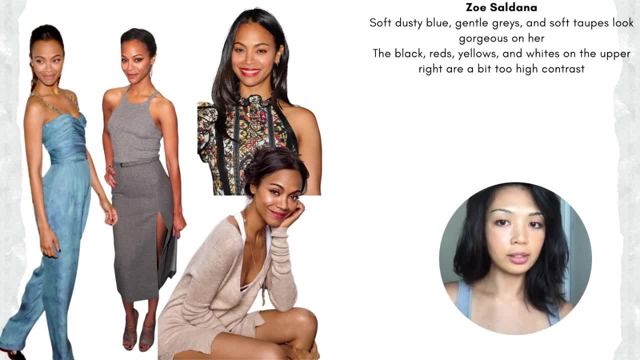 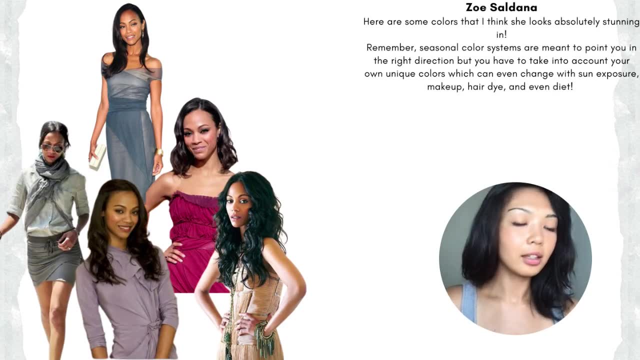 the very high contrast kind of print. it just looks very busy and just a little bit overwhelming in terms of color. and here I just wanted to finish off this video with some really lovely colors, really lovely looks on Zoe, from, you know, grays and silvers to dusty blues, dusty purples, muted raspberries and 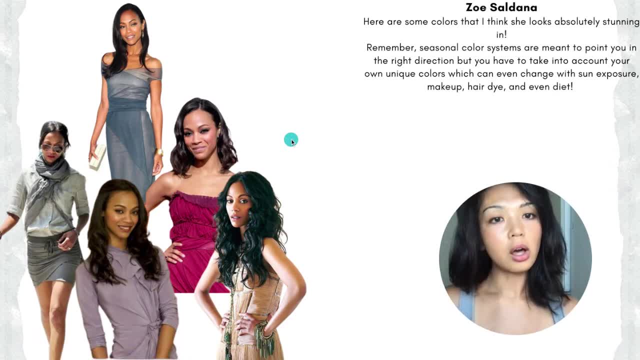 kind of cool: gray, tan, gray beiges, all really gorgeous. um, and to end again, I just want to emphasize that these color palettes are collections of colors that will probably look good on you, but you'll have to approach it on an individualized basis. some colors might work, some colors might not.